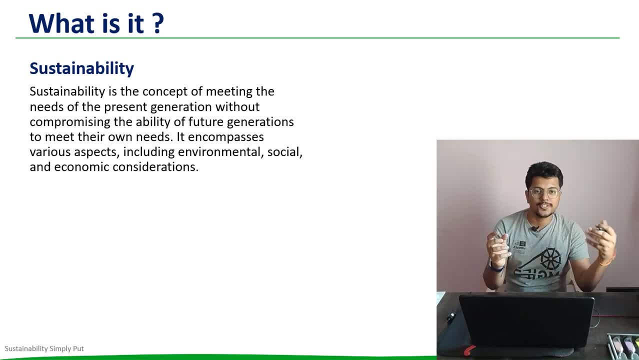 are directly associated or correlated with the energy use, right? So whatever need you take, that requires some energy, and whether that energy comes from renewable, like solar, wind, or non-renewable, means fossil fuels. So that is the question. Let's go through this. one interesting fact. 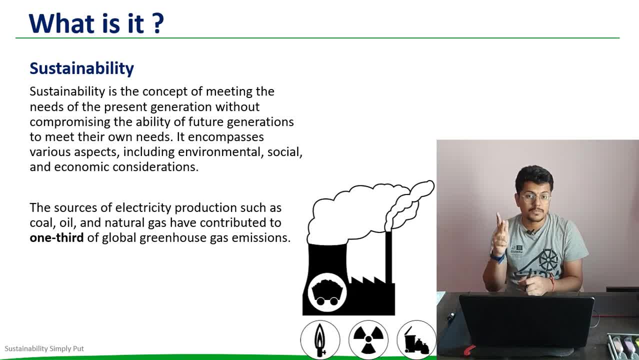 Resources of electricity production such as coal, oil and natural gas, means non-renewable sources have contributed to one third of global greenhouse gas emissions. It's 33% of overall greenhouse gas emissions that has come due to electricity production with coal oil and. 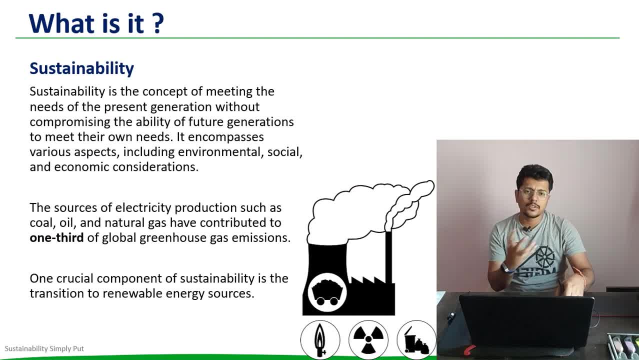 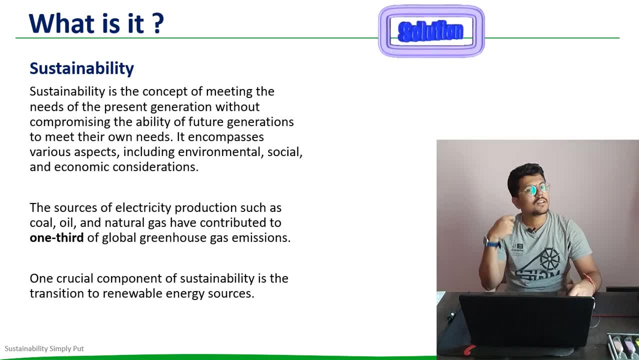 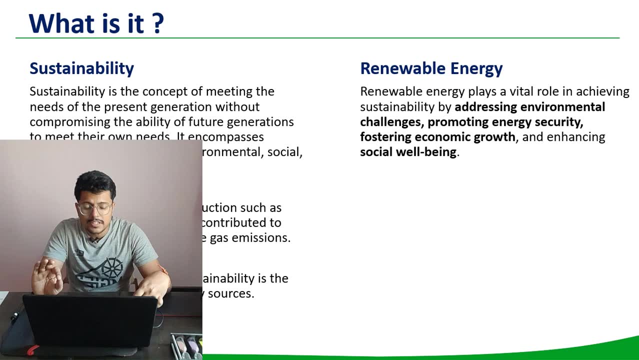 natural gas. So it's a huge contribution And in that backdrop, the role of renewable energy in achieving sustainable development, meeting all the needs, is very much important. So renewable energy does play a very vital role: addressing environmental challenges, promoting energy security, economic growth and enhancing social well-being. So how? 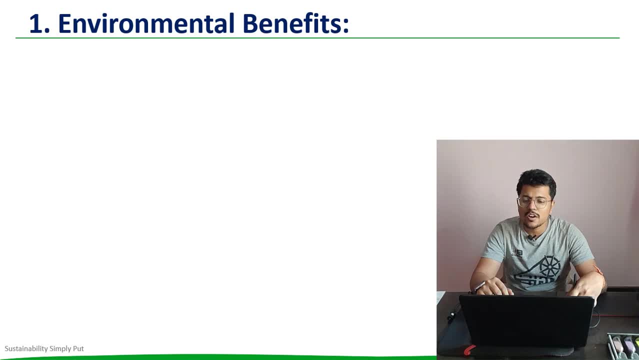 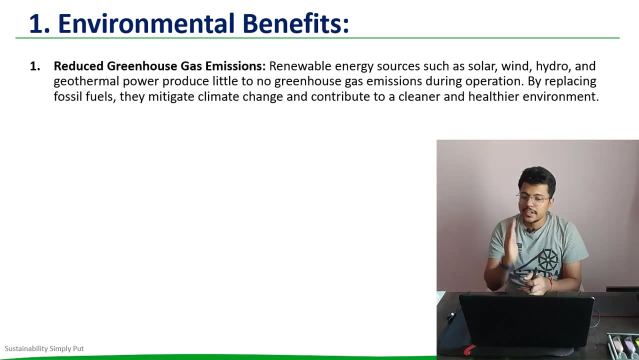 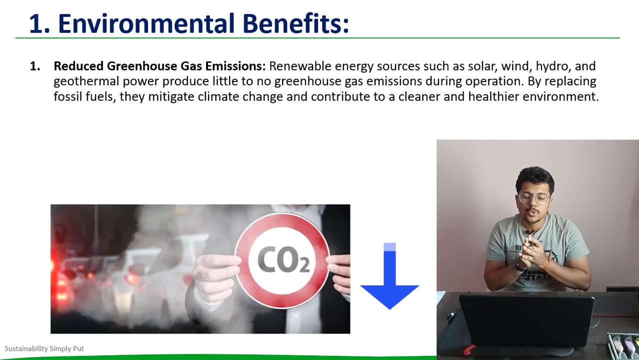 We will explore in this video in detail. So let's talk about first environmental benefits. First benefit that you can identify, that is, reduced greenhouse gas emissions. Renewable energy sources such as solar, wind, hydro and geothermal power produces little or no greenhouse gas emissions during operation. So by replacing fossil fuels, we 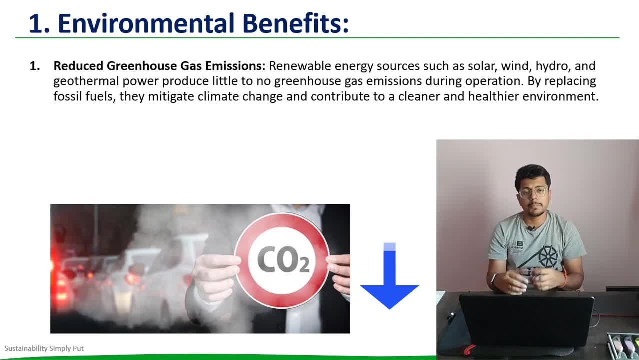 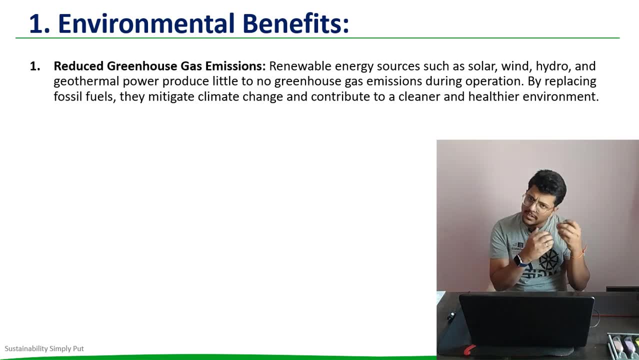 can reduce the greenhouse gas emissions. So here some people might ask that: what about the solar panels? What about the waste generated by solar panel, or turbines in the case of wind? So what about it? Let me tell you, if you analyze overall life cycle thinking don't. 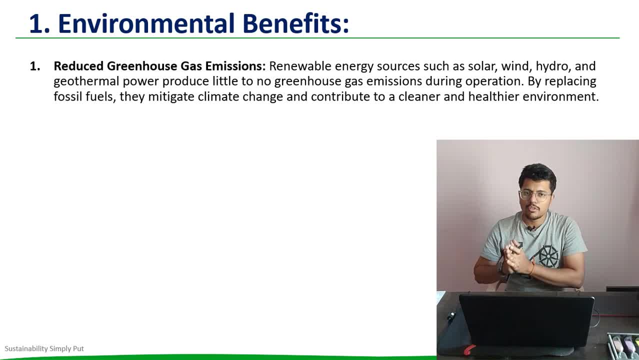 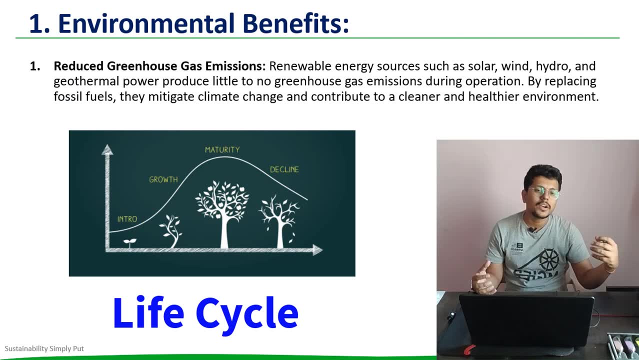 you think that you have to look from the cradle to the cradle, from scratch, from where it comes to the point where it becomes waste and where it has zero value, as we say right, So it disintegrates into the nature. So you have to identify, you have to think through. 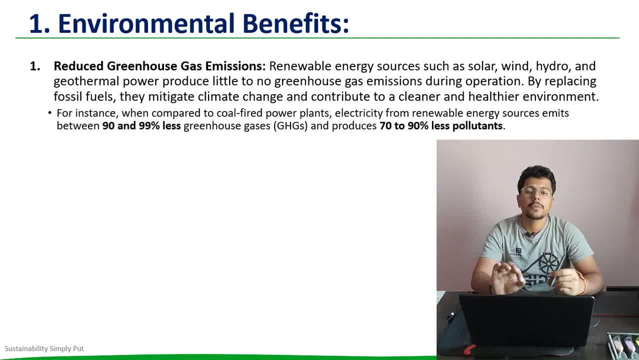 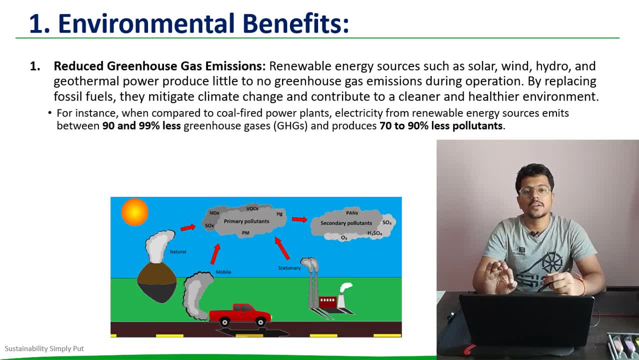 life cycle aspect, life cycle thinking. Compared to coal-fired power plant, the electricity produced from renewable energy sources Amid 90 to 99% less greenhouse gases and produce 70 to 90% less pollutants. So isn't it great? So your GHG greenhouse gases are also less. The other pollutants are also less. 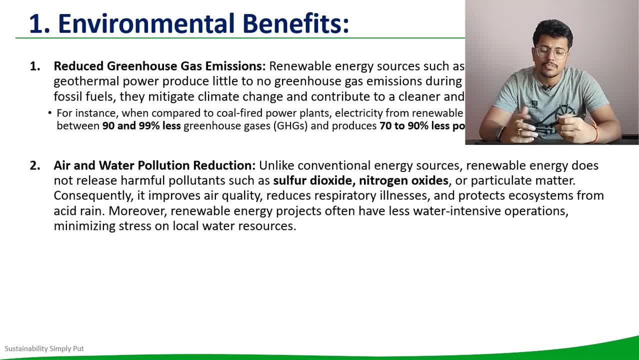 Second is air and water pollution reduction for the conventional energy sources, So maybe coal or maybe gasoline, petrol, diesel, So they emit the pollutant. These are also greenhouse gases, For example sulfur dioxide, nitrogen oxides and percarbonate, So they emit the pollutant. 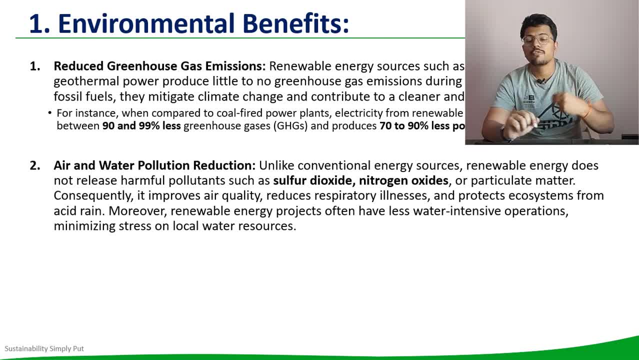 These are also greenhouse gases, For example, sulfur dioxide, nitrogen oxides and percarbonate. organizations put CO2, nitrogen oxides and percarbonate on their fuels to manipulate energy, which is harmful for health. Through this, if you are shifting towards renewable, 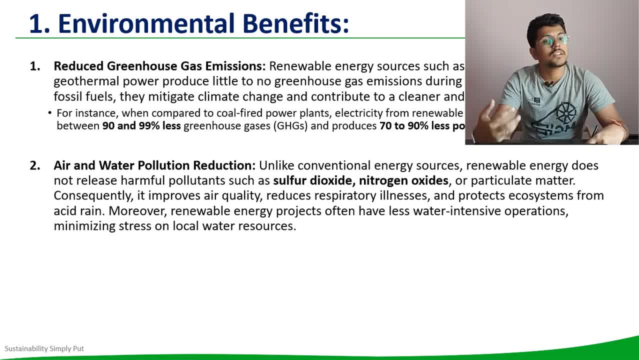 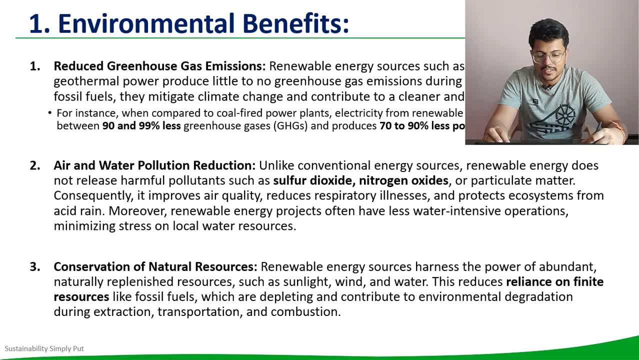 energy, the overall health of the society will also improve. So isn't it great Conservation of natural resources. Renewable energy, which is abundant in nature, can replenish itself, and this reduces reliance on products like fossil fuels. Geddy Amar, nurturers of fossil fuels. 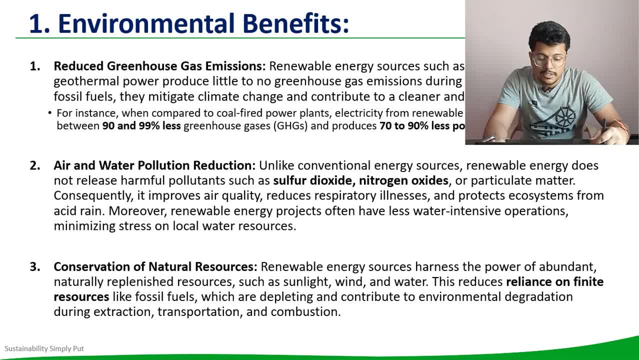 Auchi Keppri夠 be. I don't have energylandsge traditional marshal airborne benefits like enva. you will stop or reduce the environmental degradation, uh, during extraction, transportation and commission point to note is when we use non-renewable sources. so let's say: 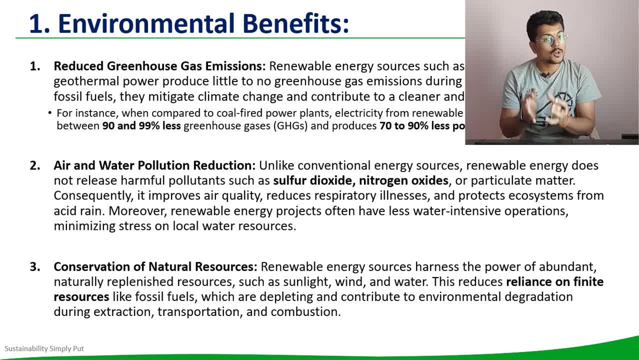 for example, we are using petrol or diesel. okay, it's not only about the combustion, it's right from the extraction of the gasoline, right, then the transportation, then the use, the combustion and the required machinery to operate all these things. so we have to consider all these aspects. 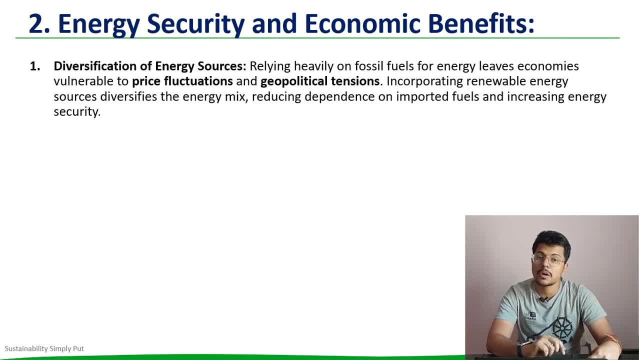 as well. let's move to the second level of benefit, which is about economic. first is diversification of energy sources. if, as a country, as a society, we are heavily relying on fossil fuels, what is the damage? so it leaves economies vulnerable to price fluctuations and geopolitical tensions. 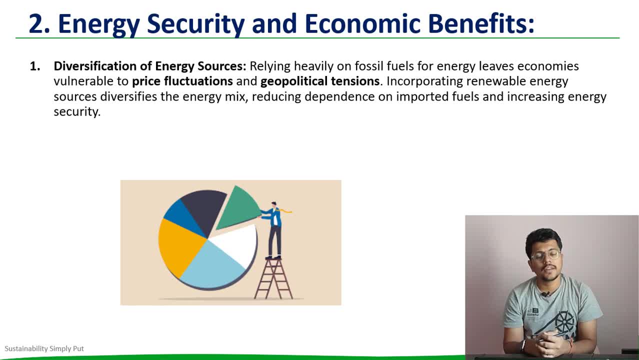 the second level of benefit, which is the global economy. is the global economy we are talking about- and that is when we are talking about the global economy we are talking about, like as a country- is there any kind of economic development? there is an economic purview. so you will find that whenever there is a 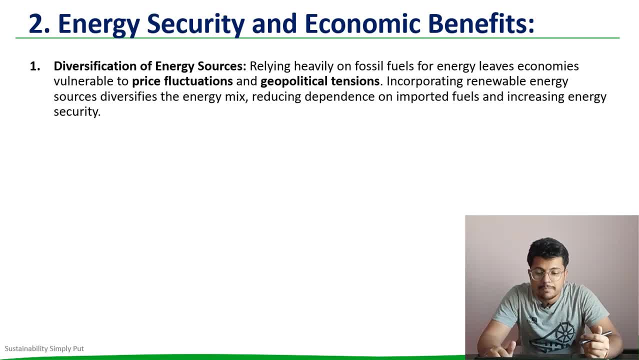 geoeconomic confrontation, geopolitical confrontation. there is oil or there are fossil fuels or there are energy issues, right, uh, maybe rare earth, metals or the. for the society, for example, diversification means if our 20 percent energy is coming from fossil fuels, then another 20 percent can come from solar, 20 percent wind, 20 percent geothermal and 20 percent 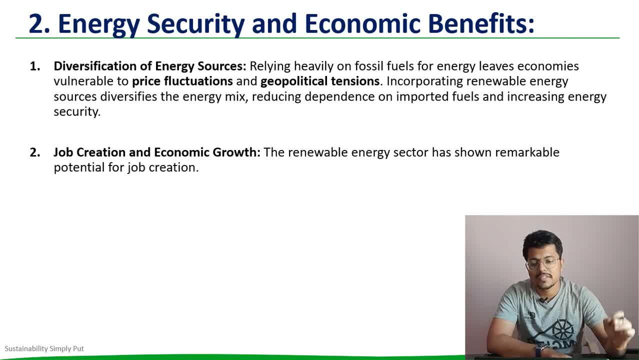 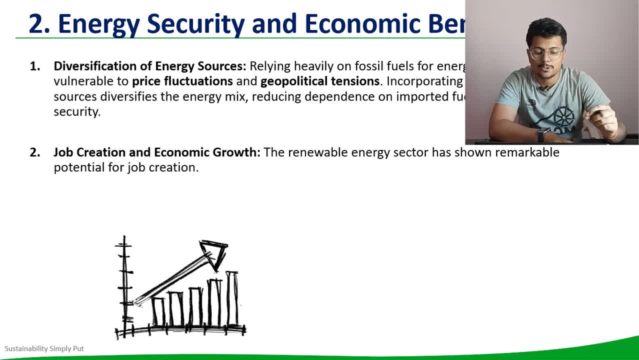 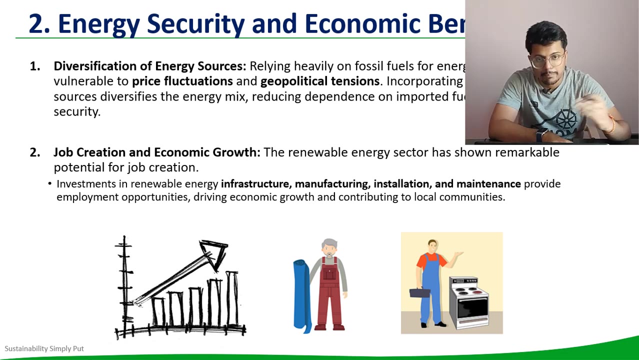 may be tidal right, so that that will be a balance of energy. then the second is job creation and economic growth. the renewable energy sector has shown remarkable potential for job creation. for example, investment in renewable energy. when we talk about it, so it it is an infrastructure manufacturing, installation maintenance, so it has provided more jobs compared to non-renewable. for. 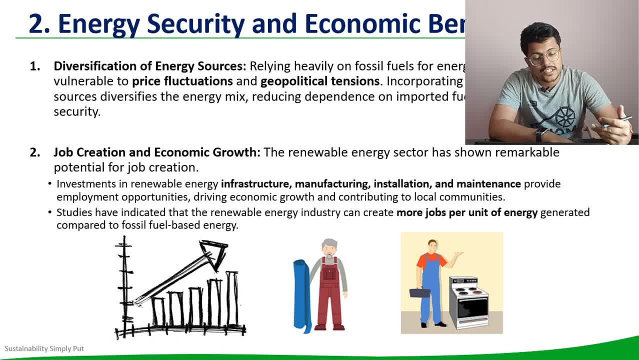 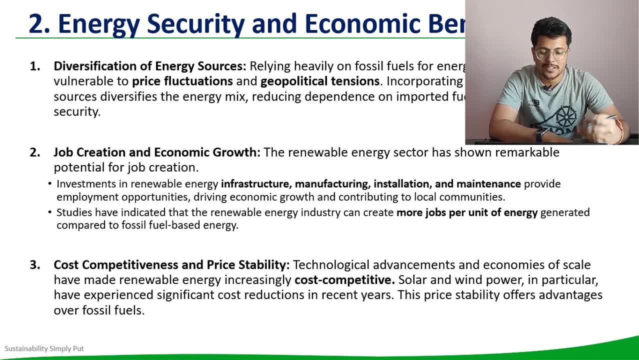 example, studies have shown that renewable energy industry can provide more jobs per unit of energy generated compared to the fossil fuels. so it's it's a really positive thing to focus on renewable energy sources. third is cost competitiveness and price stability. if you analyze the trend for last, let's say, a decade or 10 years, 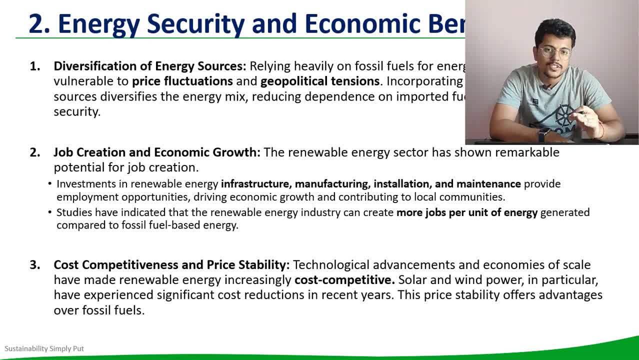 you will find that wind and solar energy have competed with the non-renewable energy sources as well, so it's really cost competitive. the price has stabilized and it also gives organizations or companies benefit because now they can have the solar plant and they can- they can sell this energy. 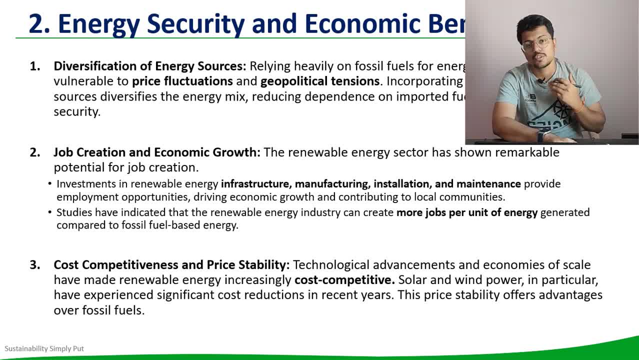 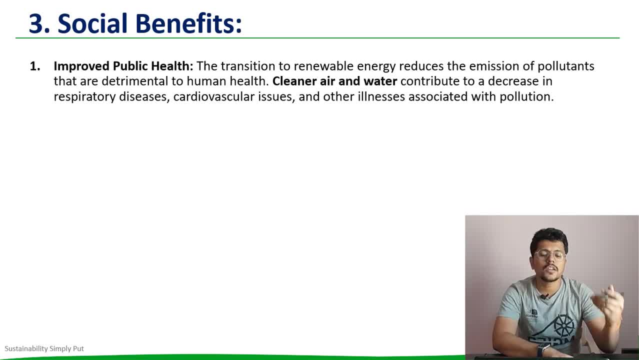 grid as well. so this is economic benefit for them for the long term future. let's move to the third tier of benefits, which is social. first is improved public health, and it's very clear that if you have clear air, pure air, pure water, then definitely it is going to improve the health and with the 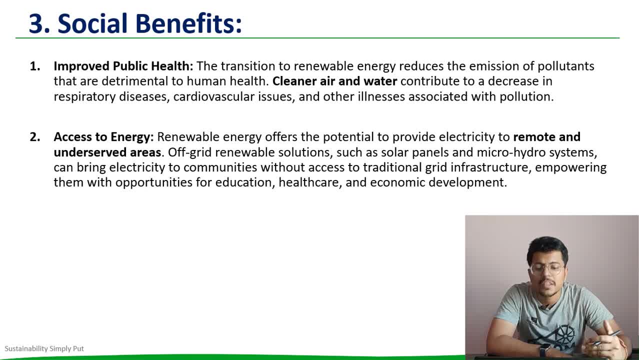 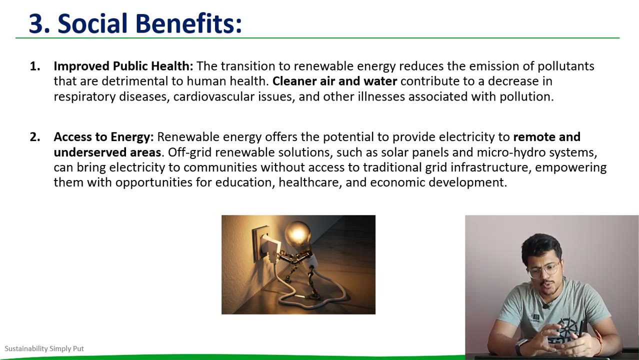 renewable energy sources. definitely you are reducing pollution, you are reducing harmful particulate matters, so, yes, it is good for health. second is access to energy. renewable energy offers potential to provide electricity to remote and underserved areas, for example, area where conventional grid infrastructure has not reached right. so at that point also, you can provide the 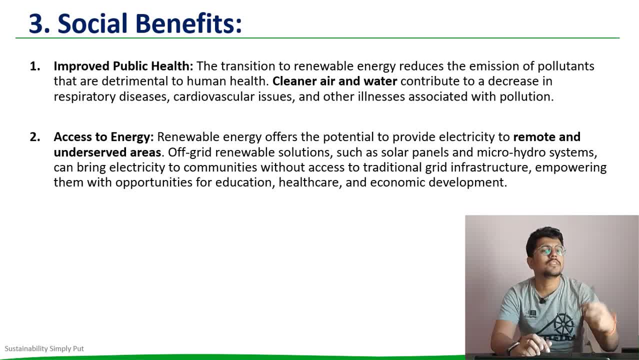 energy, uninterrupted energy supply, and which will good for the overall society as well. for let's let's take one scenario. why do you think there are all corporate offices, all the businesses in cities? only why, because they have the better electricity supply, better internet and network supply right, and that's why business is there. so what if we could provide the electricity? 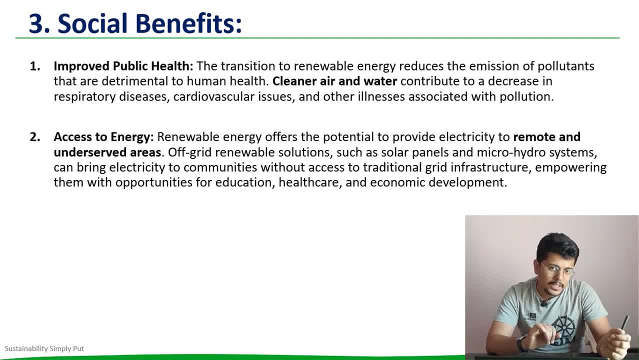 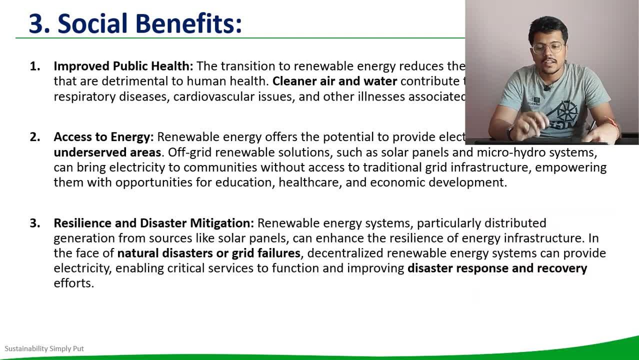 all the basic infrastructure, maybe internet support in a rural area so that people can work from that place as well? right, so isn't it empowering people? third is resilience and disaster management. you might have seen that after any flood or cyclone, we require almost 10 to 15 days to resume the energy supply, electricity supply to these areas, and we 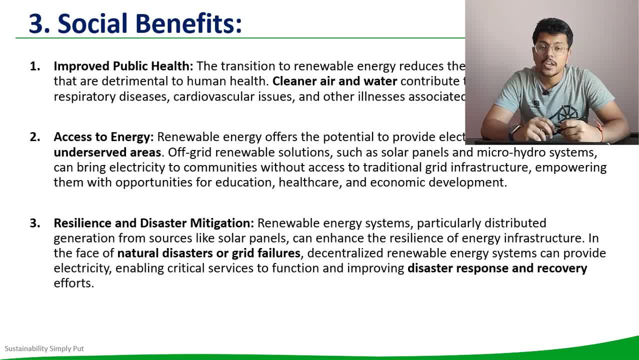 have seen that many times when such kind of disaster happens, so it can hamper the critical areas like hospitals. so in that case, if we are having distributed energy generation units like solar and wind, so the end result is such a simple but veryлекto now also in terms of what the characteristics of renewable energy support for some offices. 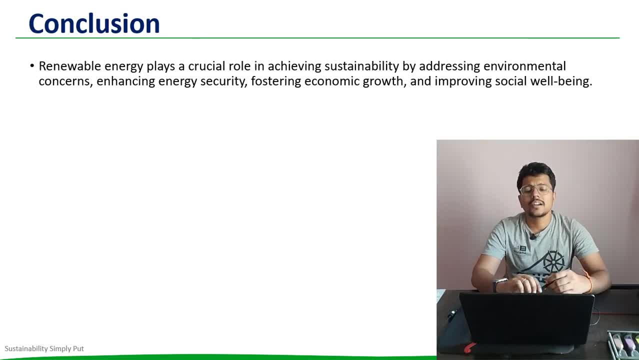 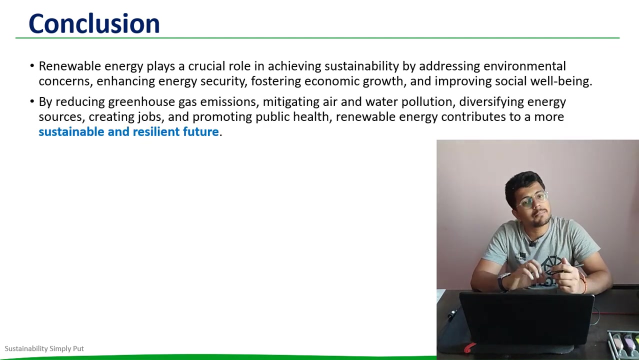 i think we can implement properly whatever is ready. for Now i would say, you know, Renewable energy- heat is much extremely important for coral andoma and, most importantly, clearly maintaining the blurred owe value of power today our energyalı. it can mitigate air and water pollution, diversify energy sources if we want. 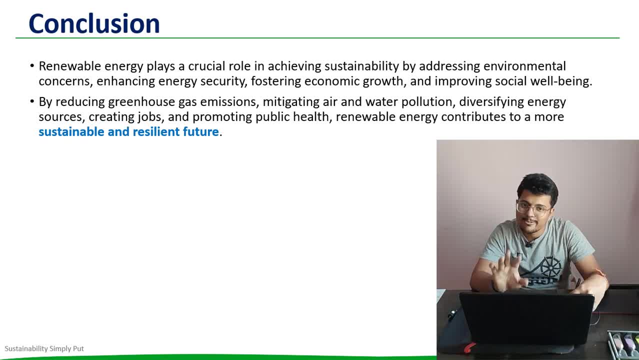 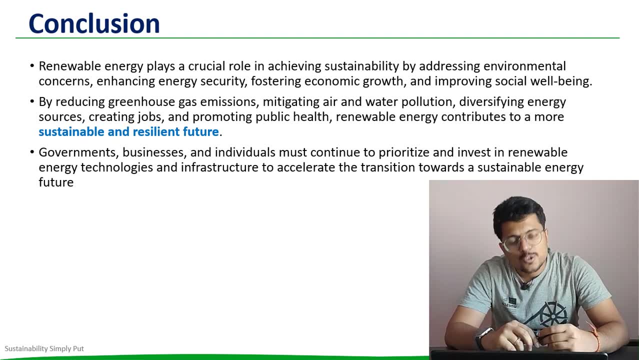 sustainable and resilient future, then renewable energy is something where we need to focus, and that's why government, businesses and individuals like us should prioritize the use of renewable energy into our operations, into our day-to-day activities, how much we can incorporate it, how much we can support. 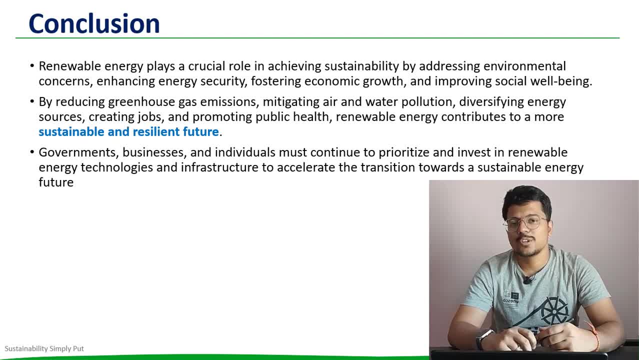 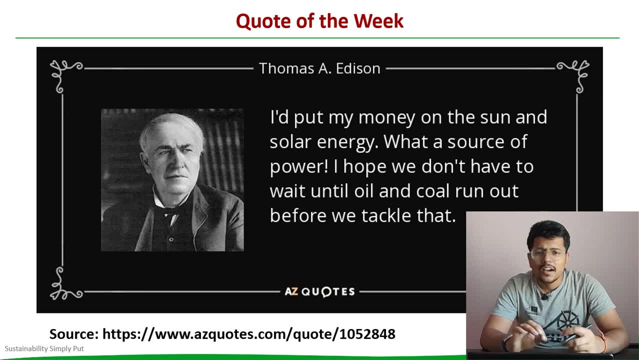 renewable energy. so thank you so much for your time. and before ending this video, let me leave you with this quote from Thomas Alva Edison. let me just read: I would put my money on the Sun and solar energy. what a source of power. I hope we don't have to wait until oil and coal runs out before we tackle that. so 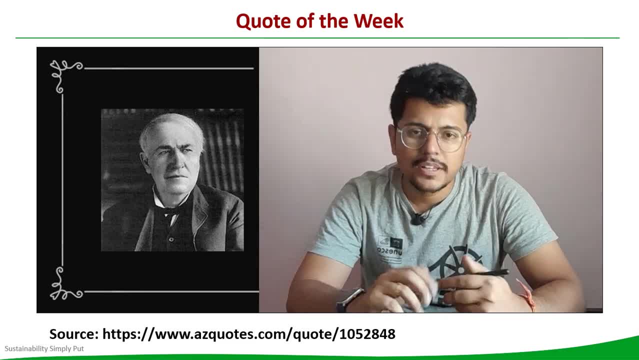 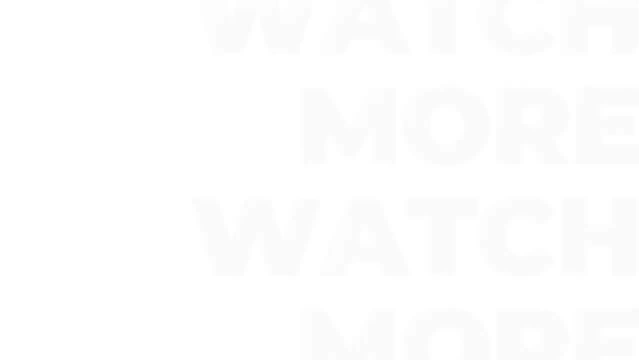 with this thought, I'll leave you over here. please like, comment and share this video. do subscribe to stay connected. thank you so much. have a great day.